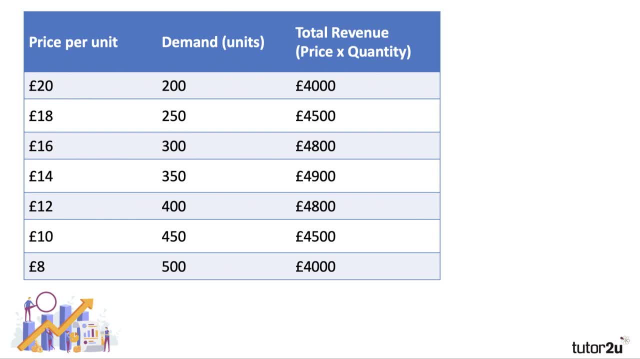 Let's look at the data. So we sell 200 units at £20, gives us a revenue of £4,000.. If we lower the price to 18, we sell 50 more. So 250 times by 18 is £4,500. 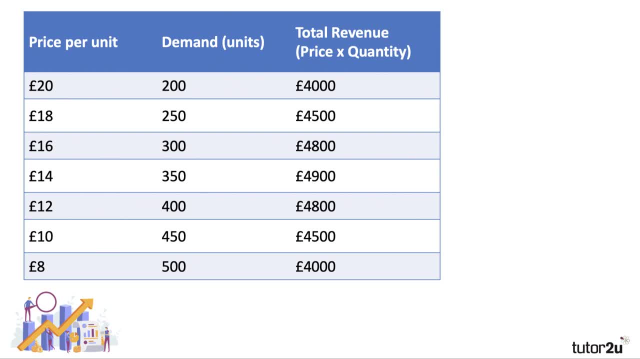 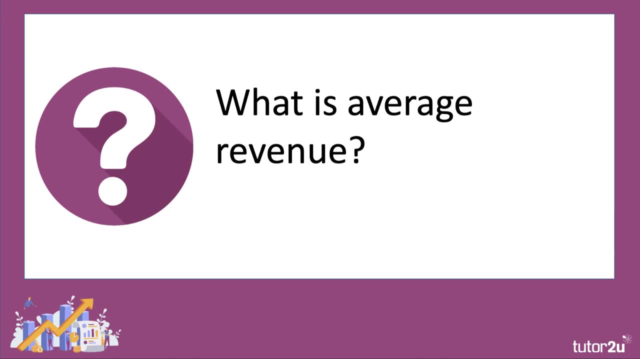 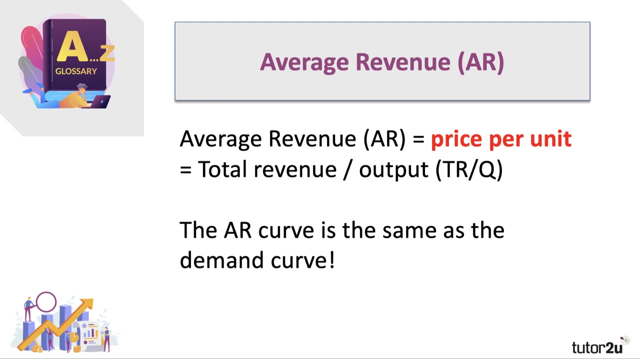 You can see what happens to the total revenue of the business. The second concept is average revenue, Revenue per unit And, as I've just said, the revenue per unit is also known as the price per unit. Simply take the total revenue, divide by the output, TR divided by Q for output, We get price per unit. 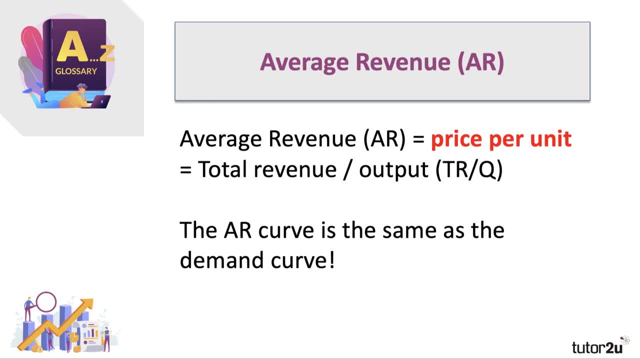 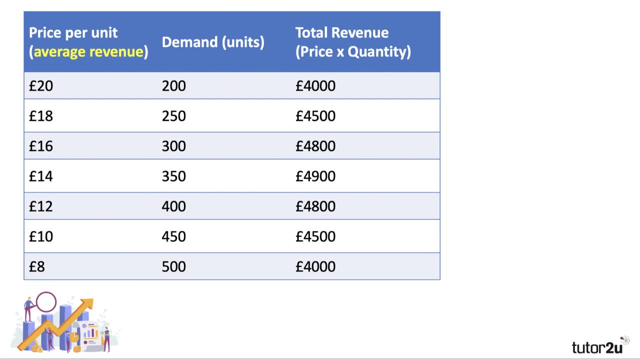 Well, in fact the price per unit is basically the demand price relationship. So the average revenue concept and curve is the same as the demand curve. So the left hand column there from the table before I've just put in average revenue same as price per unit. 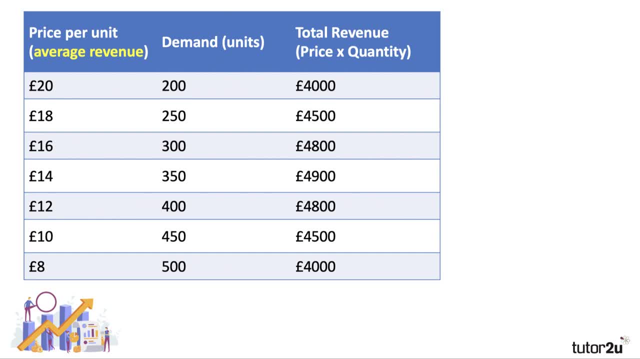 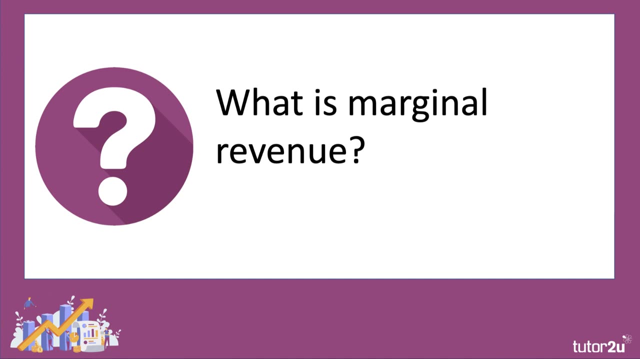 So the first column is average revenue. The second column is the demand at a given price. The third column there is the total revenue, price times by quantity. Okay, the third concept in this video is marginal revenue. Well, what is marginal revenue? 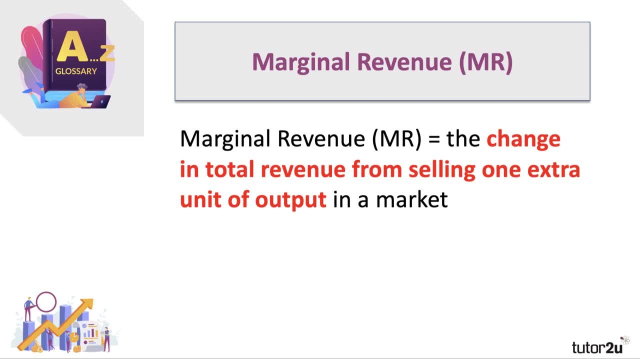 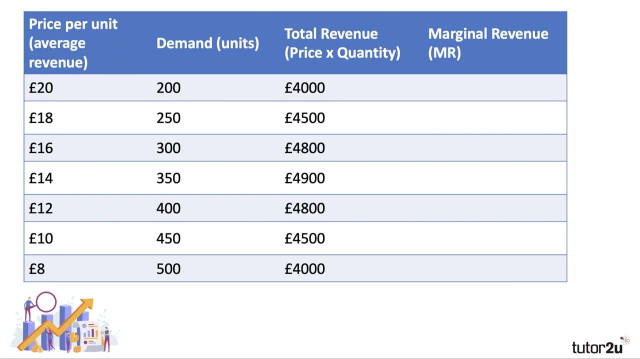 Well, it's the change in a firm's total revenue from selling one extra unit of a good or a service in a market. So if you have an extra unit you sell. what's the impact on the total revenue of the firm? Let's go back to our table, our example. So we're cutting the price by £2 per unit and demand is going up by 50 units. 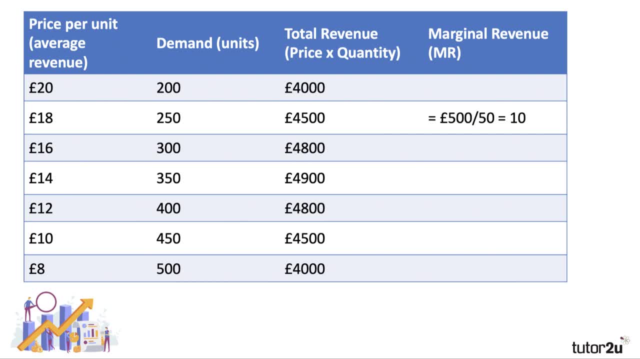 Let's take the first example here. when we cut the price from 20 to 18. Our revenue goes up by 500.. We've got column 3.. We've sold an extra 50 units. We've sold an extra 50 units. 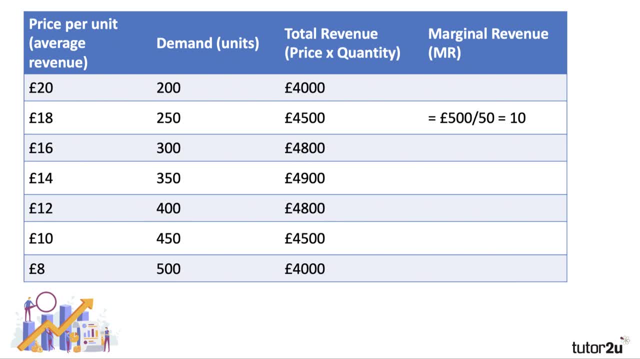 We've sold an extra 50 units, So we're getting 10 extra pounds per extra unit sold. Hopefully that makes sense. We've sold an extra 50 units. We've added 500 pounds to revenue, So our marginal revenue is 10 pounds. 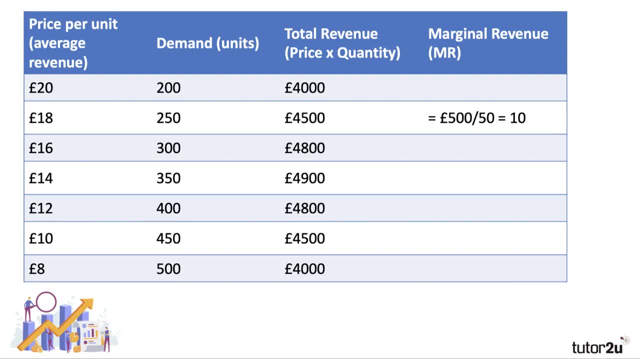 Now, if we cut the price from 18 pounds to 16 pounds again, we sell an extra 50 units, But this time our revenue only goes up by 300 pounds. So our marginal revenue is 10 pounds. So our marginal revenue this time is only 6.. 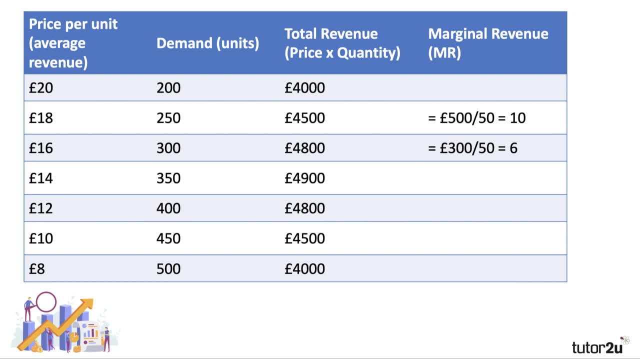 We're getting some extra revenue, but we're only going to get 6 pounds of extra revenue per unit sold And next price cut from 16 pounds to 14,. we add 100 pounds to our revenue goes from 4,800 to 4,900, divided by 50. 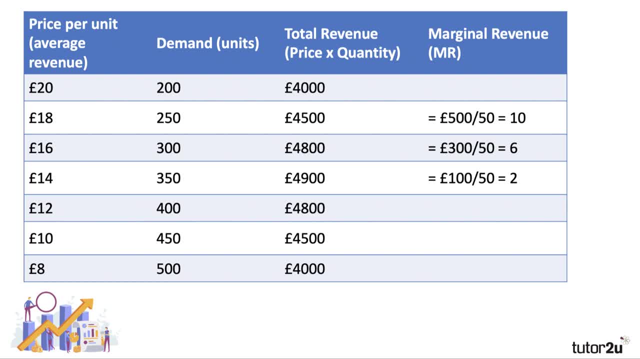 We're only getting 2 pounds extra from each unit sold. We're only getting 2 pounds extra from each unit sold. Of course the reason is we're having to cut the price by £2 on average to sell these units. Of course the reason is we're having to cut the price by £2 on average to sell these units. 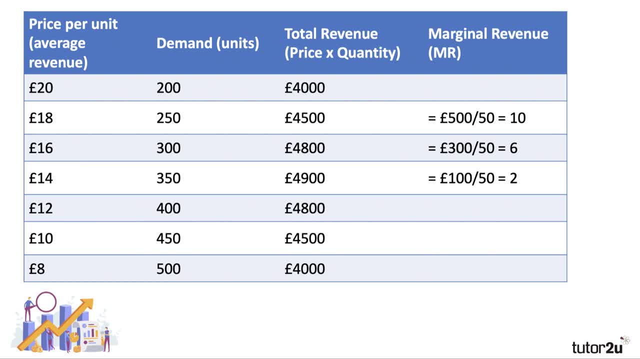 the extra 50 units. Now, thinking ahead, you should be able to calculate what's going to happen here to marginal revenue, if we now cut the price from 14 to 12.. What's going to happen? Well, revenue, of course, goes down, goes down by a hundred. 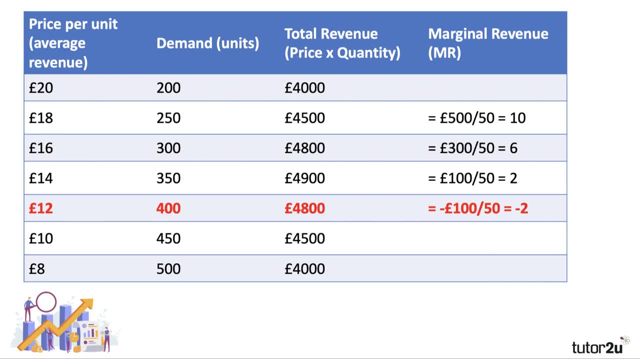 pounds. So now we've lost a hundred pounds of revenue from selling those extra 50 units, giving a marginal revenue of minus two Fairly symmetrical table marginal revenue remains negative. Our revenues are now going down. Of course the reason is to sell those extra units. we're having to cut the price to very 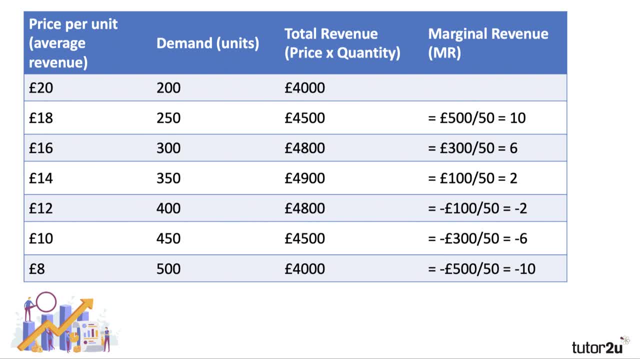 low level: 10 pounds, 8 pounds, etc. So because average revenue on the left-hand side is going down, the marginal revenue is also falling. In fact it's falling more steeply, If you can visualise that. we'll come into the diagrams in another. 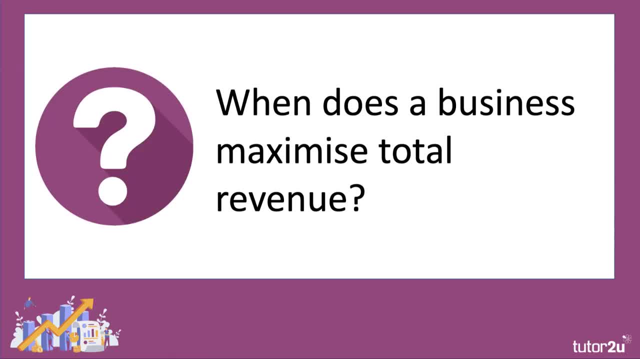 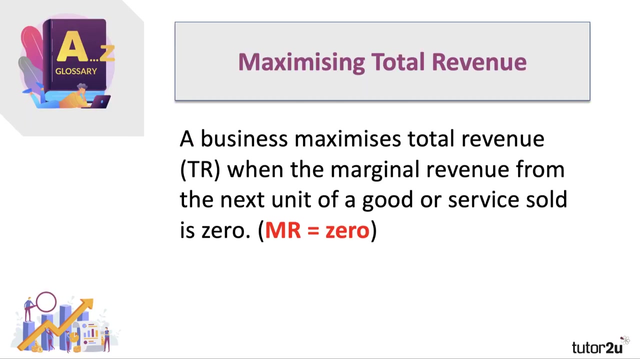 video. So where do we start? When does a business maximise their total revenue? This is a really important little idea to get a hold of, particularly as some people think that maximising revenue is a realistic alternative to maximising profit. Well, a business maximises revenue when the 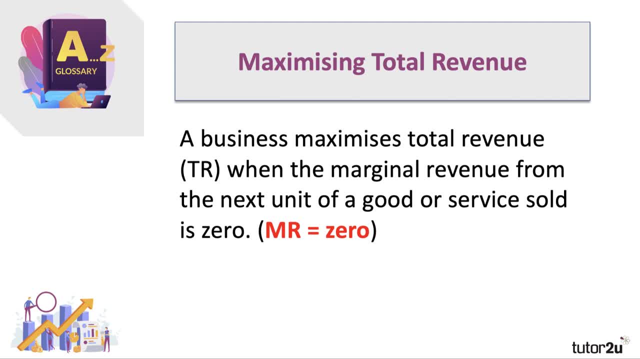 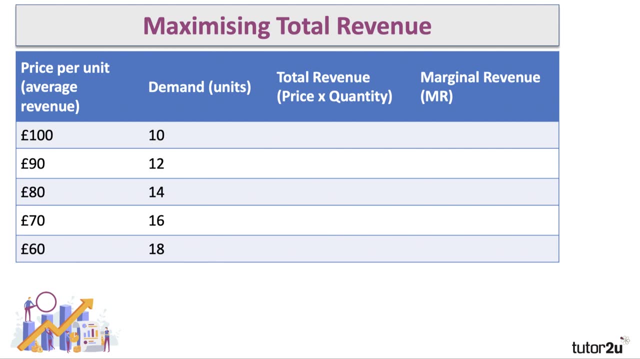 marginal revenue from the next unit of a good or service sold is zero. When marginal revenue is zero, Here's a little example. another example just to change things up a bit to show what this means. So on the left hand side we have average revenue: AR price per.